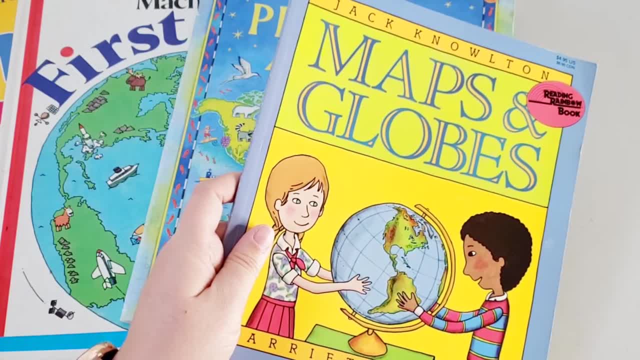 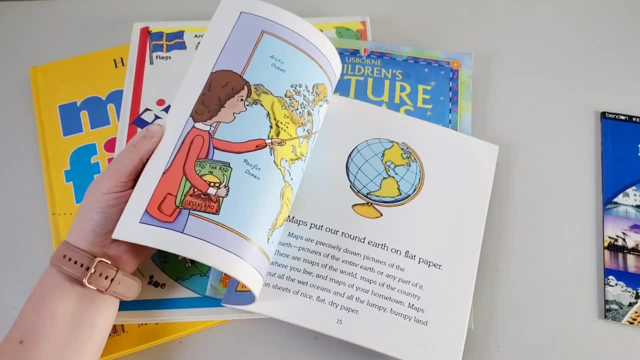 note: my husband did not know what the Reading Rainbow was. Please tell me. he's the only one in the world, Please. Okay, that broke my heart, Anyway. maps and globes. This book is literally what it says. It gives you basic information on. 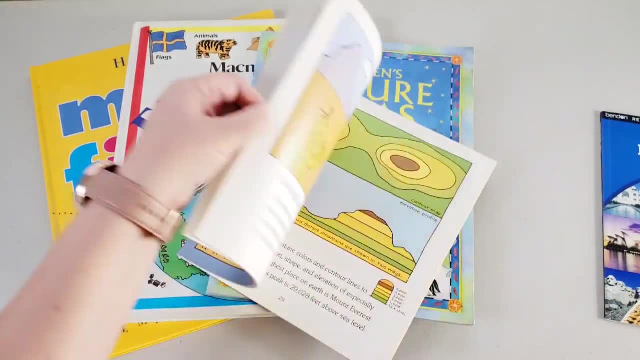 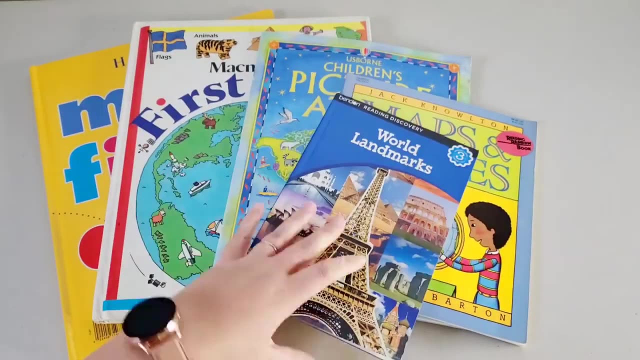 the planet and how to read the maps and traverse the planet. So really quite simple. and then this is obviously about the world landmarks- Self-explanatory. I'm not going toWarrior, but just quick snapshot and you can and see where. But 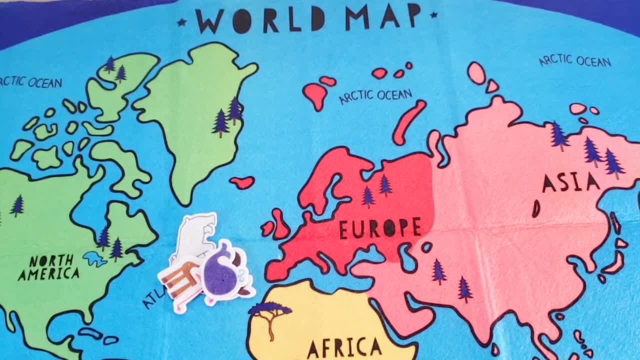 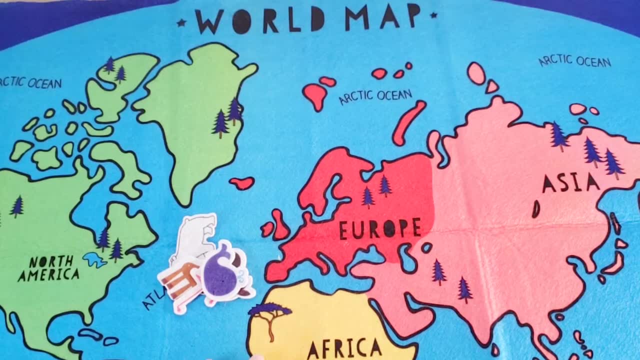 again all great references to have on hand throughout the rest of the activities. This next activity is a felt world map that I picked up from the Target dollar spot a few years ago and I believe it was $5.. Correct me if I'm wrong, but they do come out with these world maps every like back-to-school. 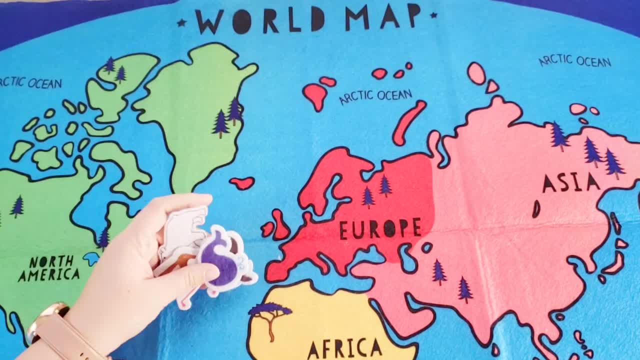 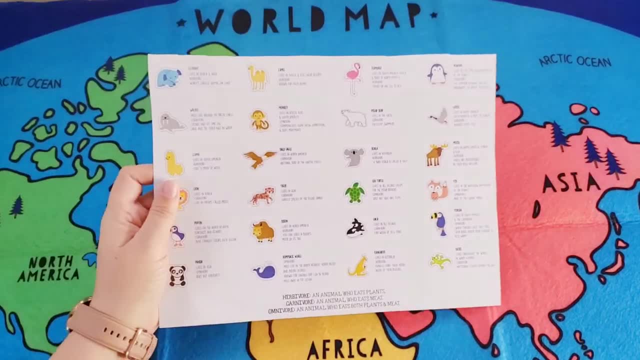 season in the Target dollar spot, so you should be able to pick them up again than what they do now. but it comes with the map itself and then it comes with some felt animals and then I kept the back of the packaging. that kind of has the key to where all these animals go, and then it also kind of has little. 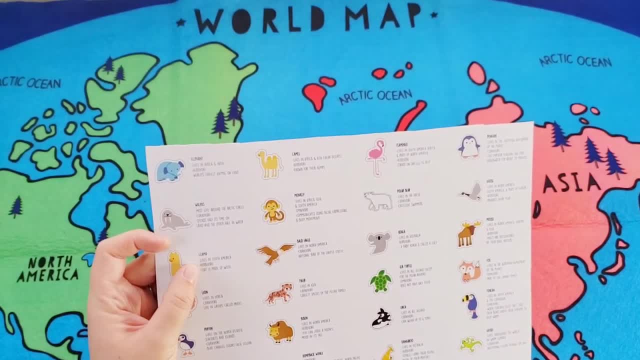 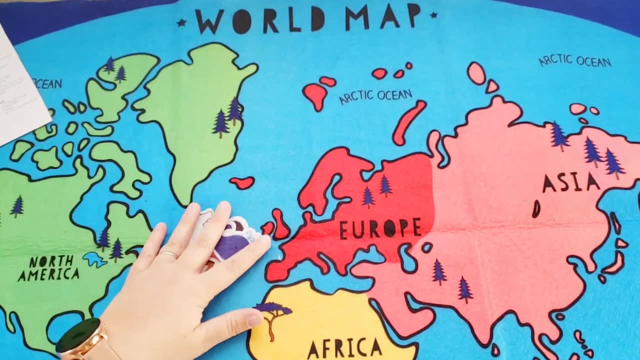 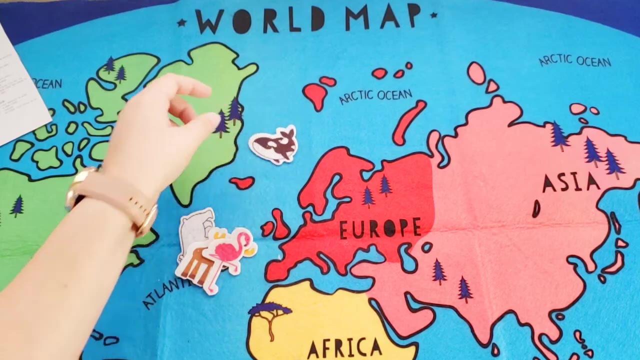 random facts as well. so the llama lives in South America, it's an herbivore and the coat is made of wool, and so that's just some random information to have on hand. and so for this activity, you'd obviously put the animals where they go, in their respective homes around the world. I'm obviously not doing this right. 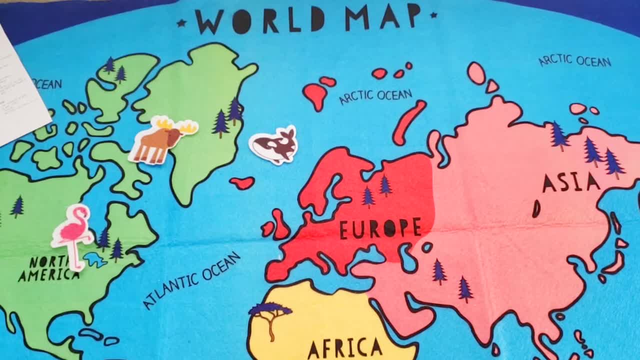 but anyway, you put them where they go, and these are actually the only animals I have. I don't know where the rest of them went and so I can't show you the rest, but that is how that activity is. you could also do this with your animal. 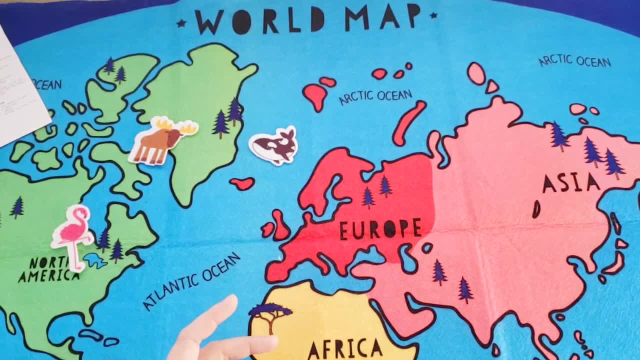 figure toys that you have. anytime you're playing with them, just discuss where would we find this animal? and do that. I've also used this map as a wall decor to have a map on our wall just of the continents. and then there's one thing that I wish I had, that I do not. 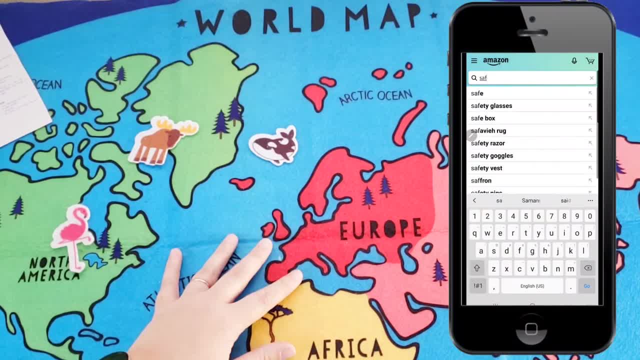 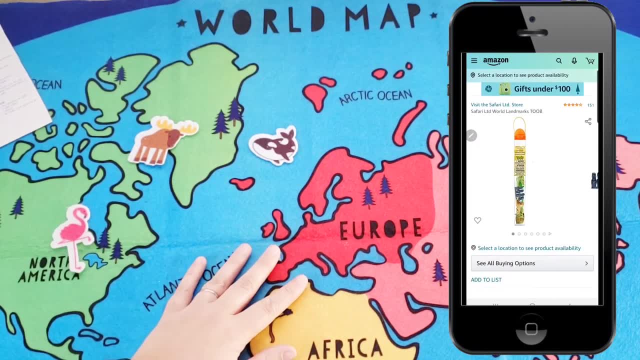 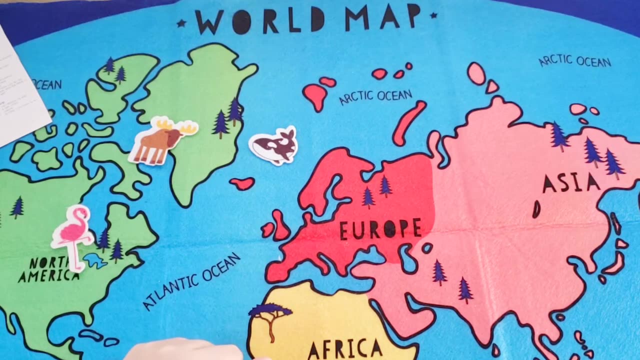 hopefully one day is the Safari LTD world landmark figures. I think this would be another great opportunity to use those and put them in their respective places around the world as well, and I'll probably bring those up again further in the video as well. but this is just another really basic. 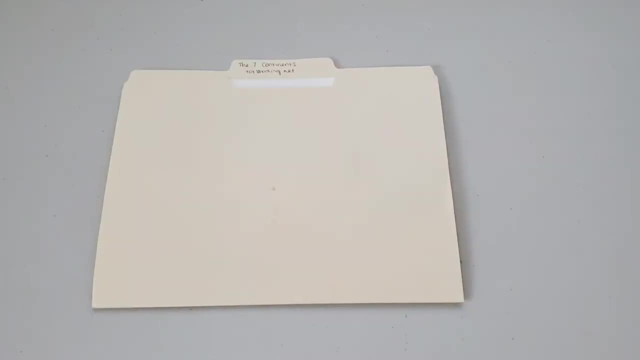 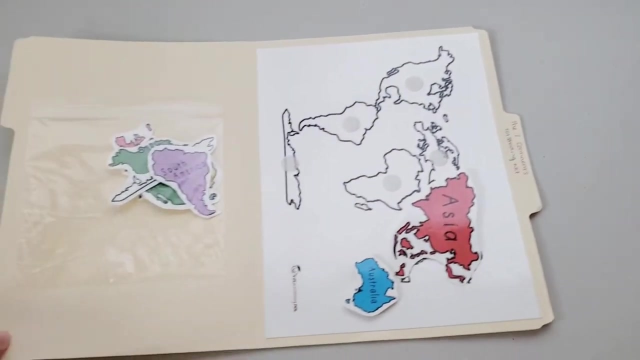 activity that you can try. next activity I'm going to show you is one I've actually shown on my channel before on how to make a file folder game, and so this is the seven continents from totschoolingnet. I'll make sure to put the printable link down below in the description box, but here is the file. 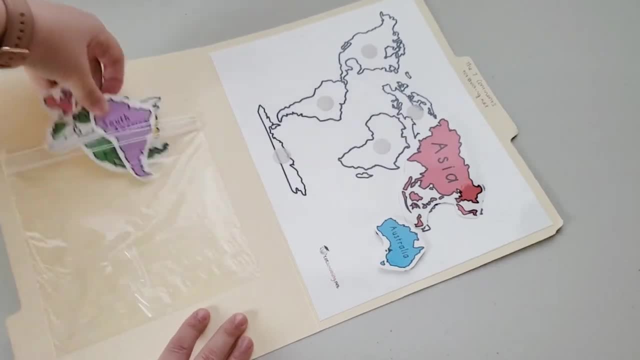 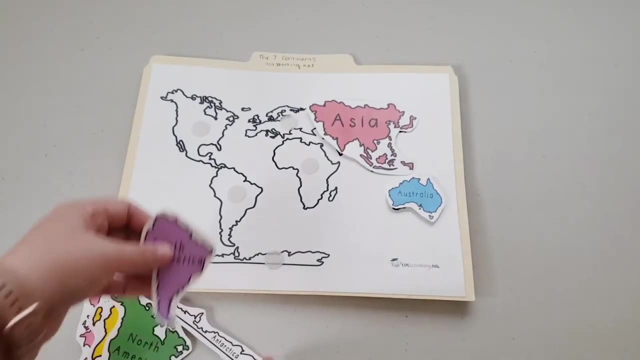 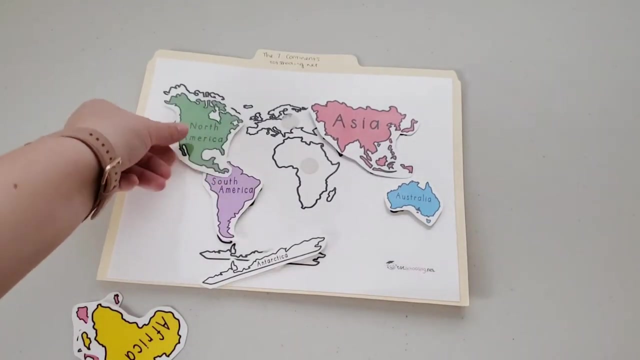 folder game, so in our ziploc bag we can then attach the pieces into their velcro places, and so this will be great for your toddler, preschool aged children, and just to match up where the continents go and have a basic understanding of where the continents are on the map, and so this is one of my 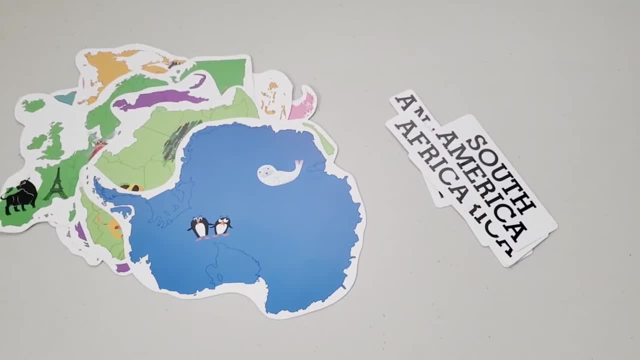 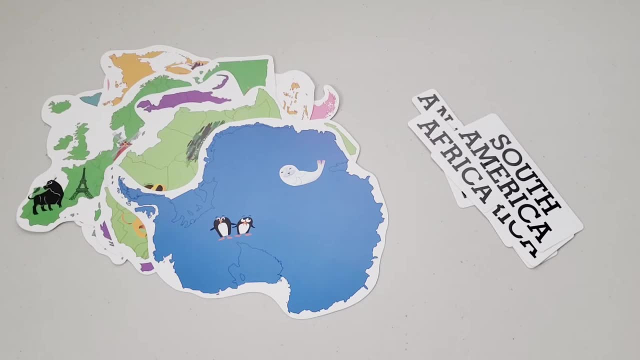 favorites for those early ages. similarly, we have an activity that I found at the Dollar Tree, but this is actually one that you could also make yourself just by printing out the pictures just from your computer, if you didn't have the resource at Dollar Tree. I got this a couple years ago maybe, so I don't know. 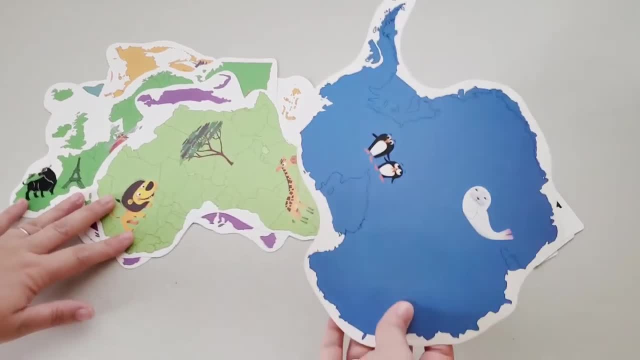 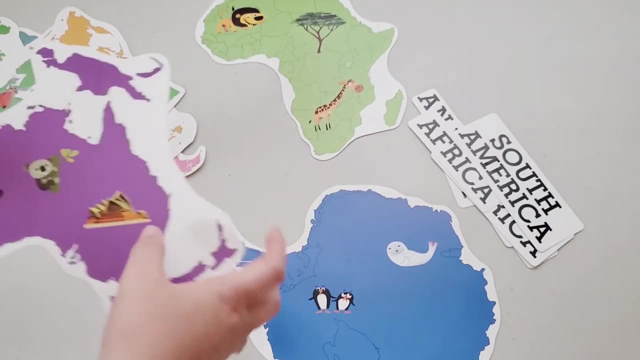 if they still have it, hopefully they should have it somewhere that they could be able to use it, do um, but they just have the continents here again with very basic of what kinds of animals you would be able to find there. um, really simple. they even have a few of the landmarks here. 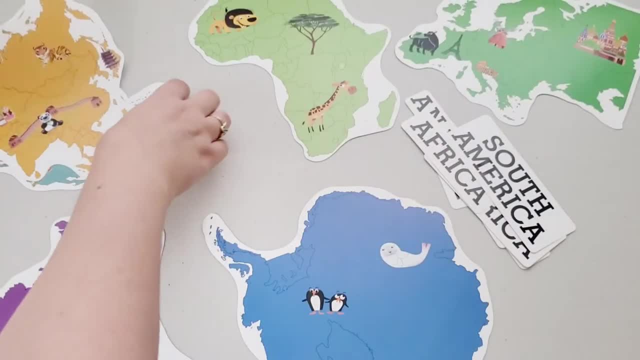 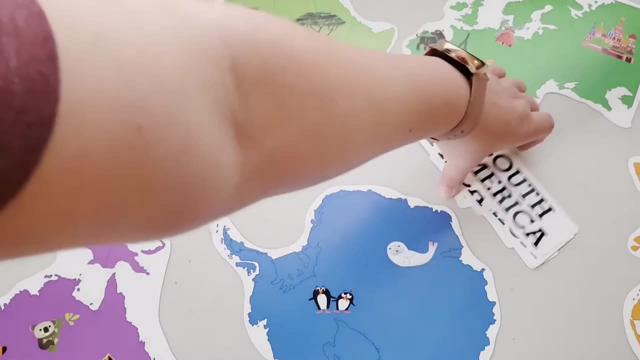 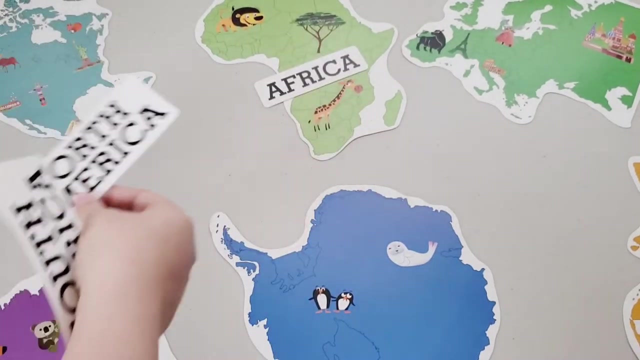 that are kind of cool, and so, again, you can just lay these out- i would even recommend not laying them out in how they are on the map- just to really make sure they understand, um, the names of each continent, and then you obviously can label them, and so this will be really fun, just to see where 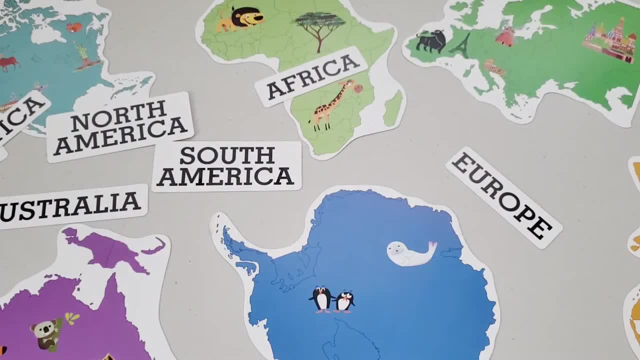 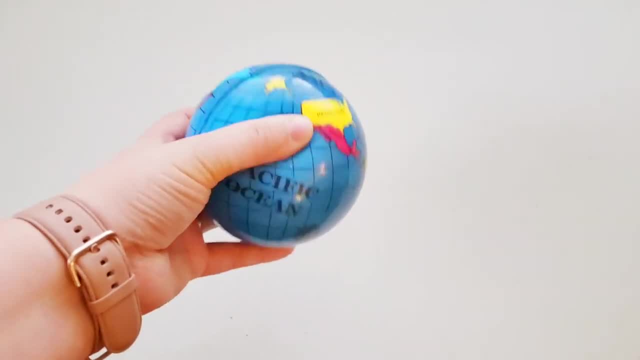 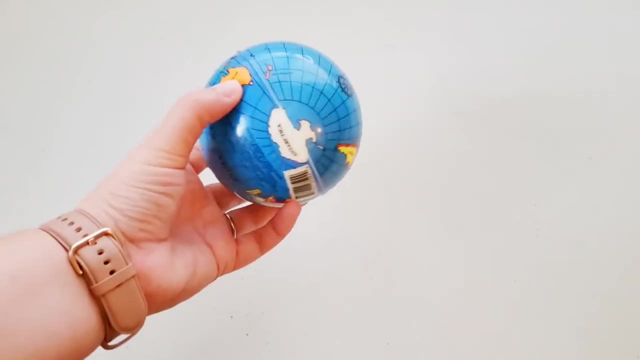 they stand um in their understanding of each of these continents. this next activity is going to use a globe little squishy ball from the dollar tree. they're there right now. i grabbed it from the stocking stuffers little section that they have, but they do have these all year round. i've 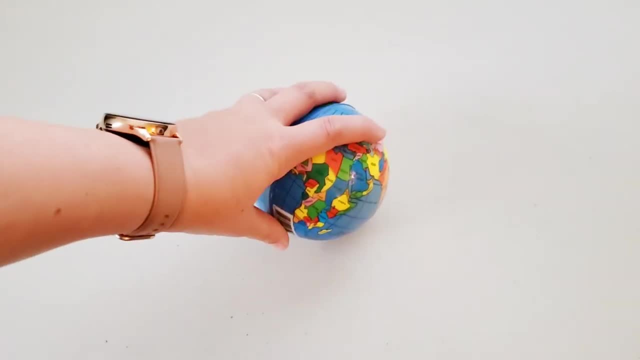 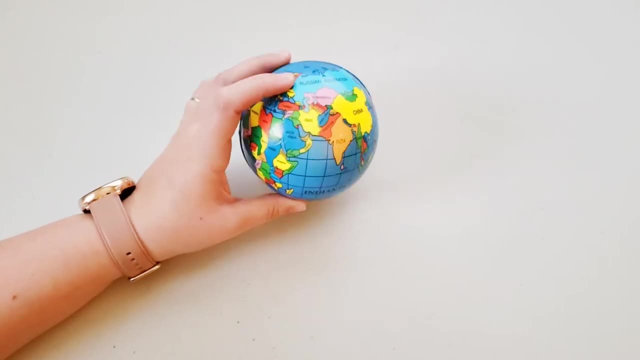 seen them many, many times, and so this activity will be a more interactive kind of activity of moving your body activity, and this will be great. for once, they have their continents down and are now learning their countries, and they're even, you know, able to be reading as well. so all 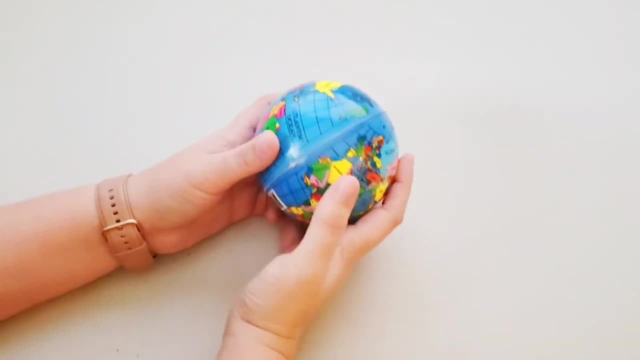 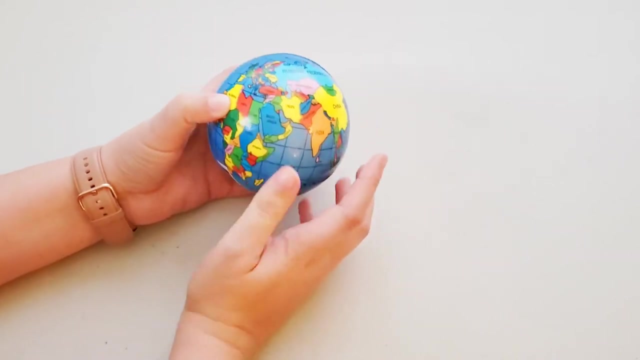 you would do is pass the ball to each other back and forth, and wherever your right thumb lands, you have to read what country that is, and then this will be great, even once they start getting older. do they know a fact about that country? or do they know a fact about that continent? i guess you. 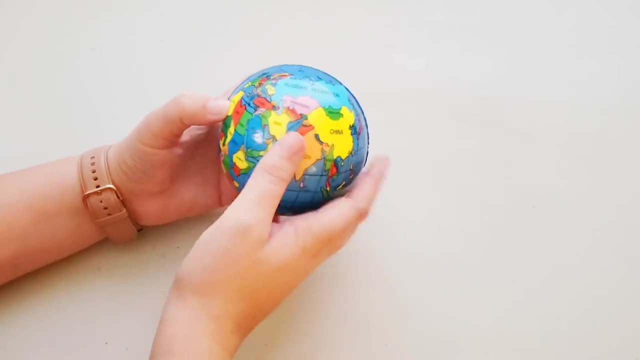 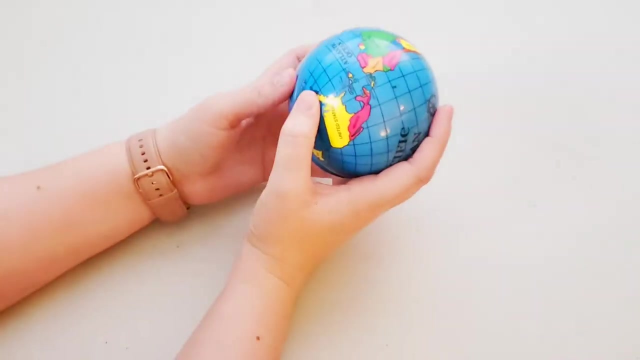 could do continents for the young people, and then you can do continents for the young people and you can do continents for the younger kids. what animal lives in that continent, or whatever the case may be, and so just wherever you catch it. um, some of them are even gonna be hard to read, even for me. 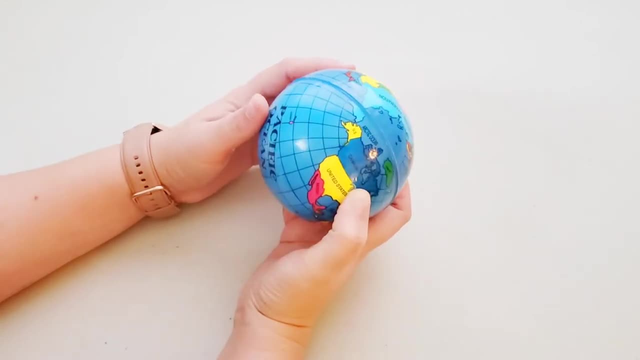 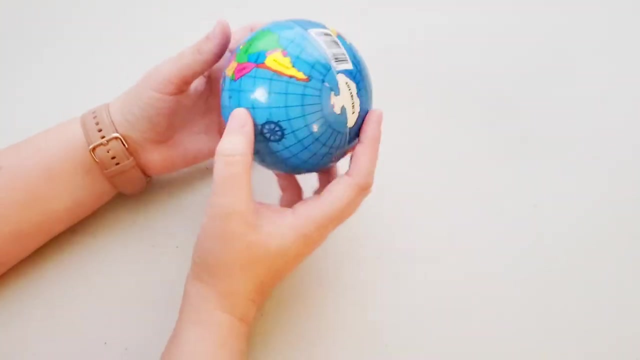 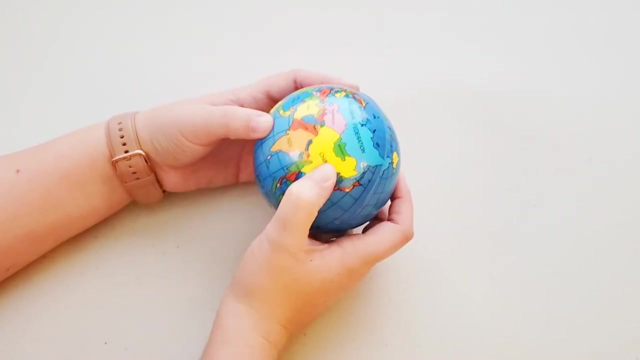 so my thumb is on canada. what information do you have about the canada? um? what does their national flag look like? um? things like that, random facts about each country or continent, depending on their? um level of difficulty. china: what do we know about china? um, so this will just 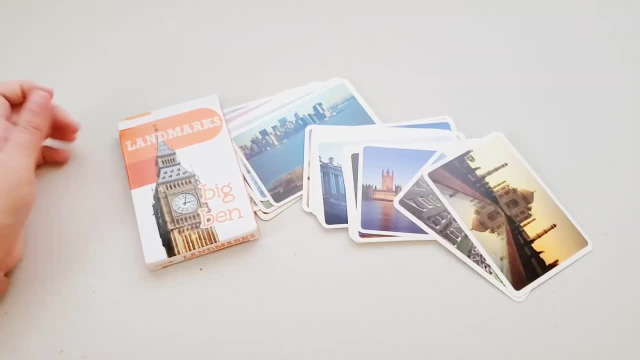 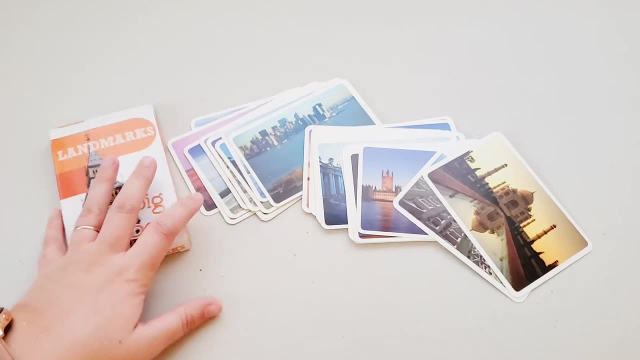 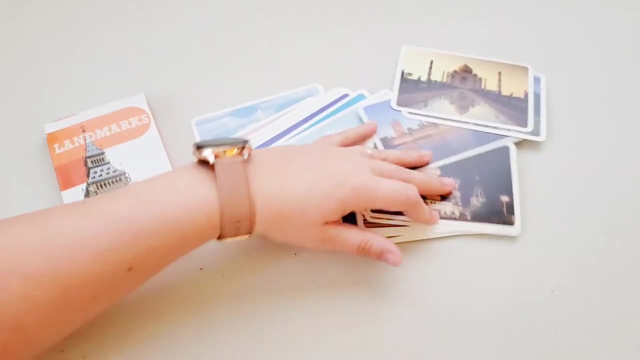 be a more fun activity to get them moving around. next we have the world landmarks flashcards, again from the target dollar spot, one of my favorite areas to shop for learning activities. this is another great resource to learn about some of our most famous landmarks and this is another opportunity where I really wish I had those safari ltd landmark figures. 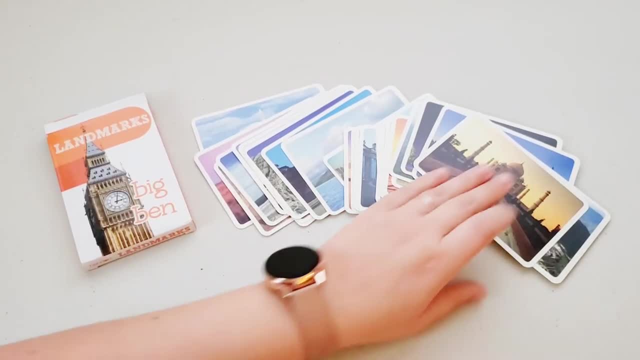 that way, we could then match them with where they go and learn about the information while we look at the آمانه مر fresco و again, Iför تِغياد مس quyيس و ، سَفَاشيْ سلهل س었어요 مجισماoned значитبه facilities and learn about the information. while we look at the. 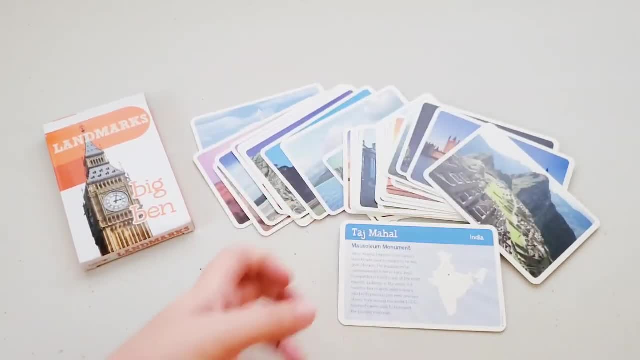 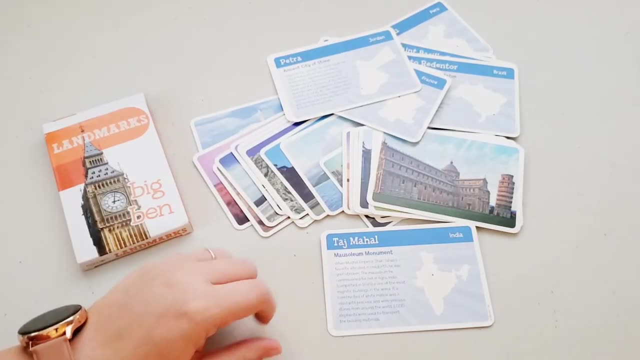 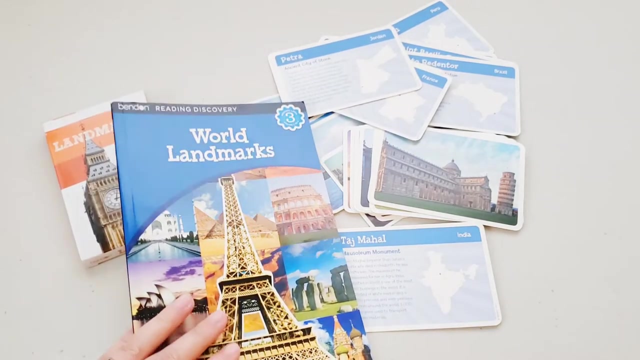 the little figures. so on the front they have a picture of each of the landmarks and on the back has all the information of where it can be found and any other information you need for those landmarks as well, and so this is a great resource if you had this and the book to go with it. even. 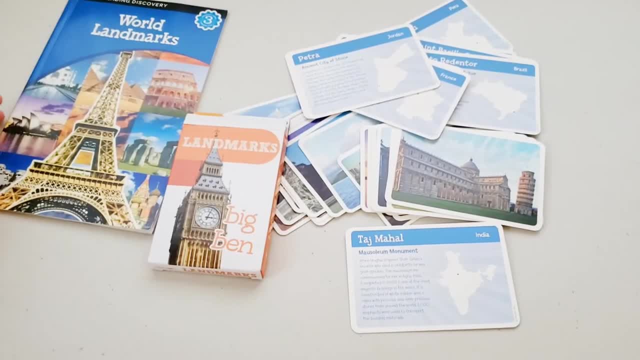 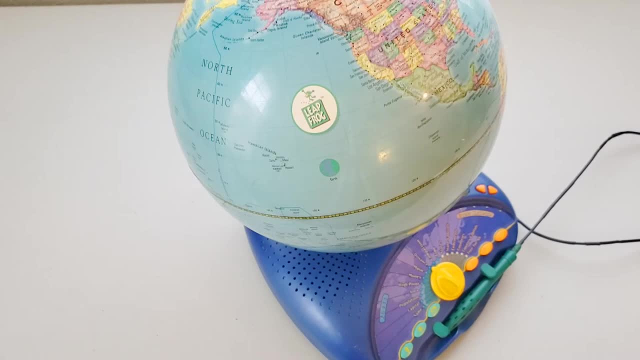 better, and then again, the more you can layer all of these different resources, the better. okay, the next resource I have for my kids is this leapfrog interactive globe. this is something I found, I believe, at the salvation army or the goodwill, only for a few dollars, and so I made. 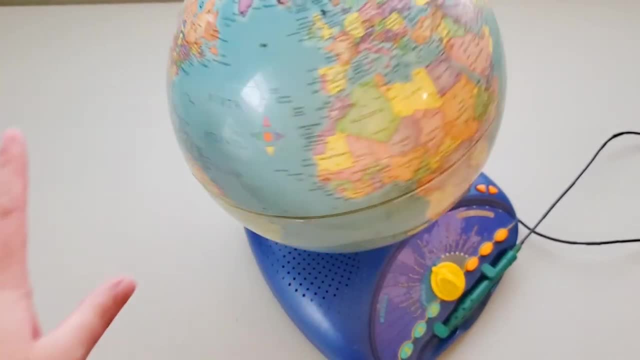 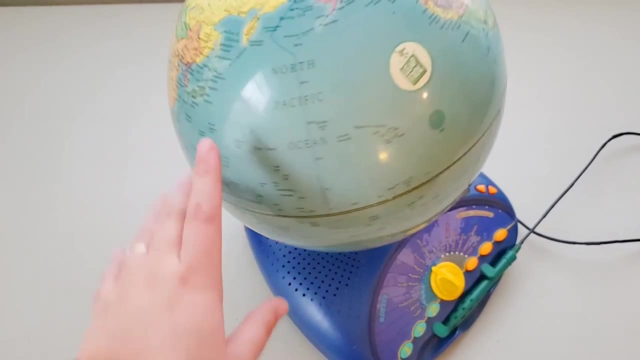 sure to snatch it, and so what it is is a globe. again, that's one of the another really great resource, just a basic globe. but this one happens to be interactive, and so when we turn it on, well, first let me talk about what all it does before I turn it on. and it starts talking because I don't. 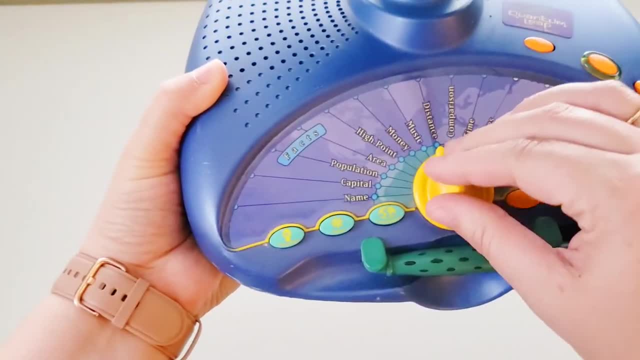 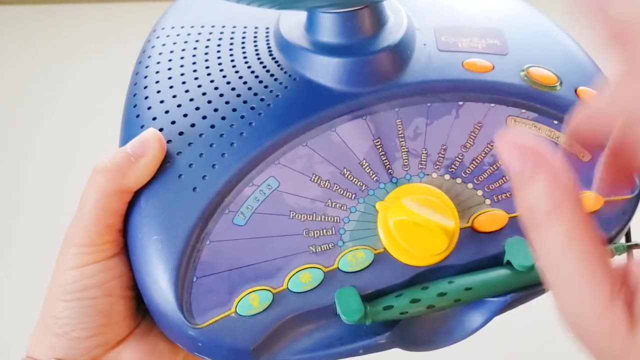 know how to do it right. so I'm going to turn it on and I'm going to turn it on and I'm going to turn it off. so on here we can turn to. we can turn the dial to whatever topic we want to talk about, so we can talk about the names of whatever it is we're talking about, the capitals population. 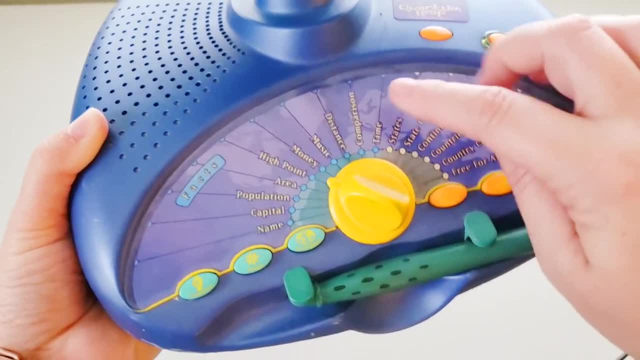 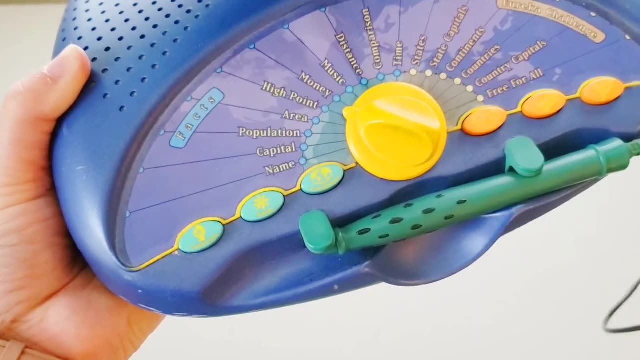 the area, the high points, money, music, distance, all of these different things, and then we can choose if we want to talk about the countries. I don't know if you can see that. very well, let me see if I can focus it better. we have the states and we have the continents, and then over 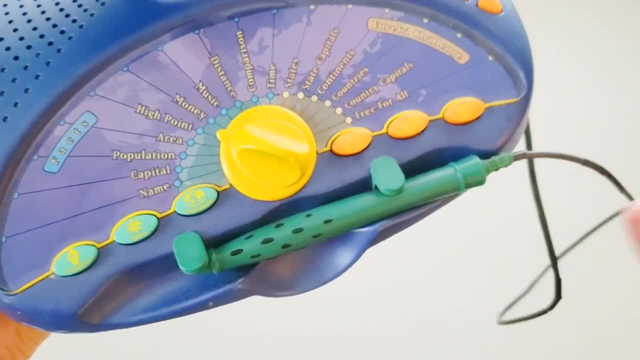 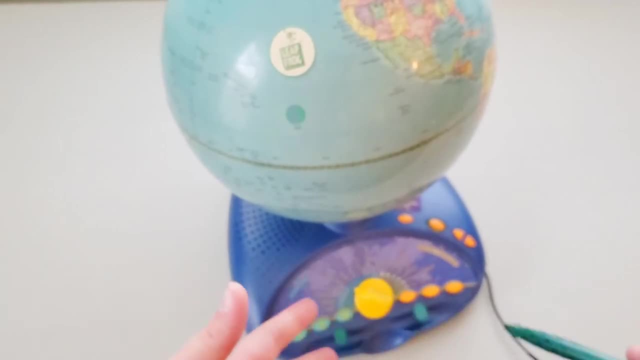 here we have the states and we have the continents, and then over here we have the countries, and then these buttons are actually a quiz type trivia game style for you to play with as well, and so it also comes with the pen. so when you're doing the quiz, hold on. let me focus it again: when you're doing 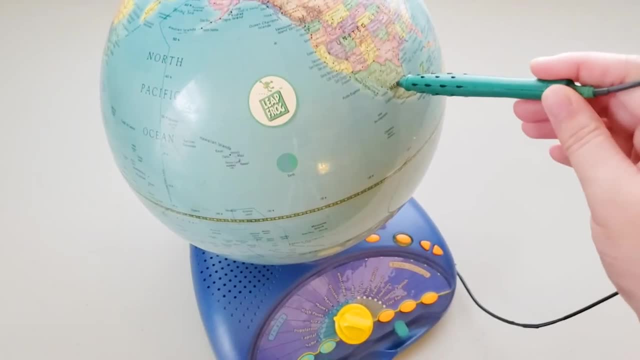 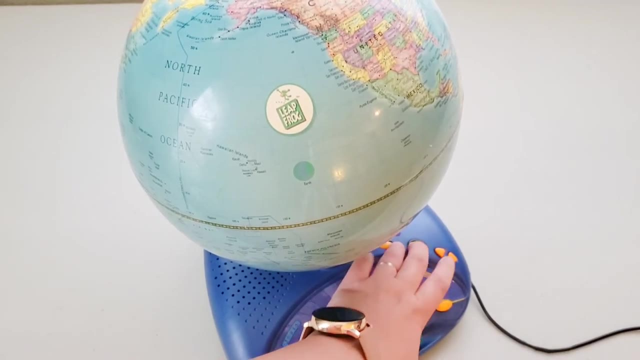 the quiz. you would then tap on whatever it's asking you to find. so Mexico is the answer. let me tap there. so let me turn it on, just so you can see, and we'll see if I can get it to turn back off. welcome to the leapfrog Explorer. 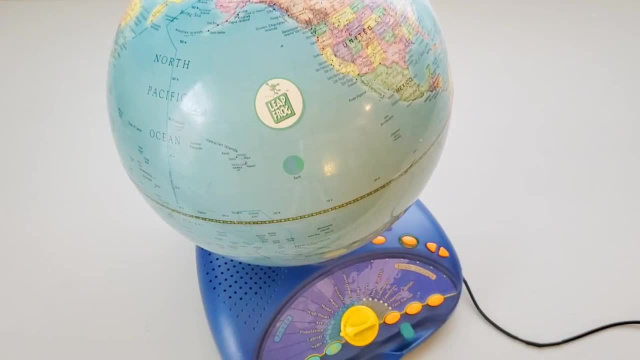 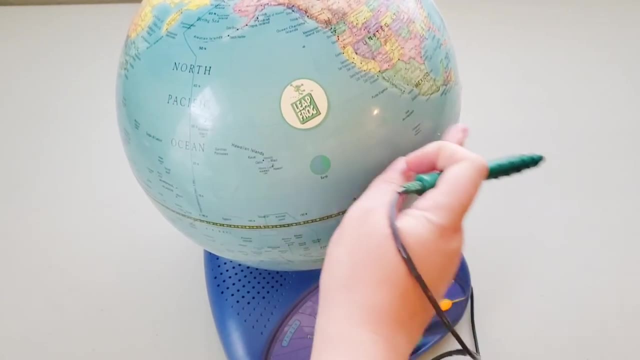 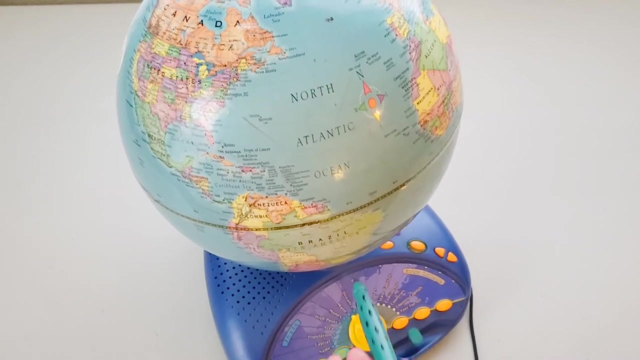 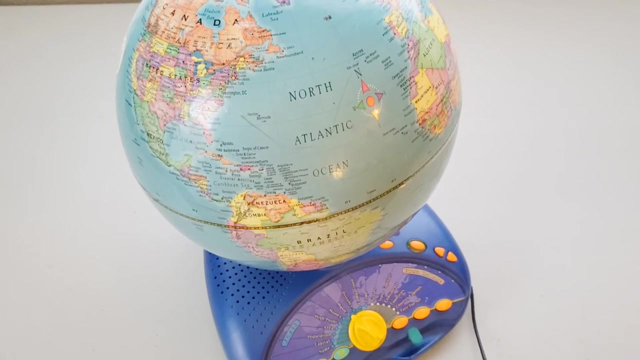 touch the globe for information, so I have put it on continents, continents. let's talk about this: North America, South America. okay, if I wanted to know about the music here, South America, music, Chile. it provides an example for us. that's really cool. now let me show you the quiz. 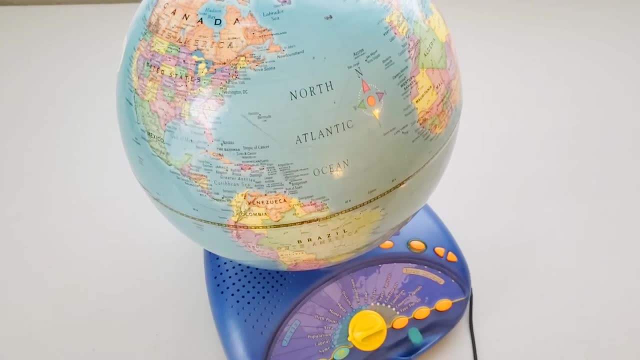 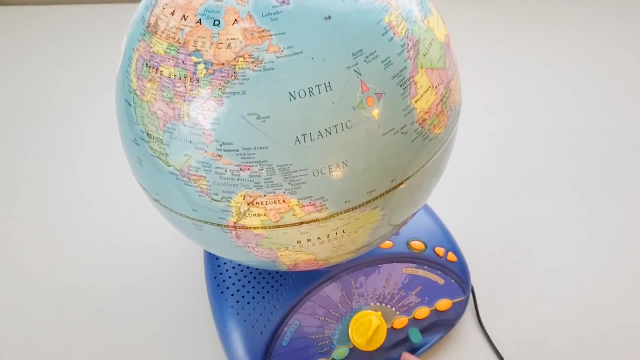 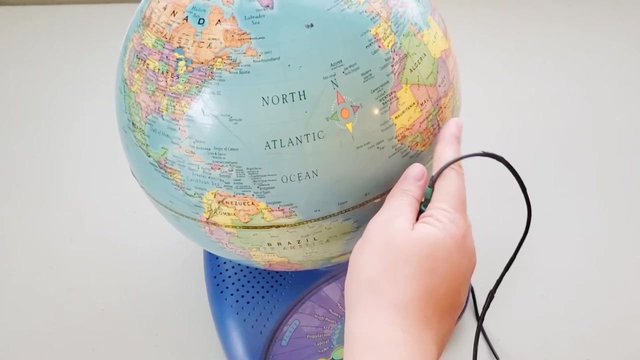 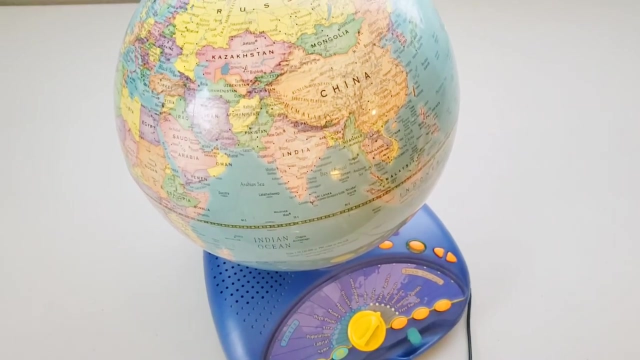 mode here to play, to play eureka. turn the dial to a game. Let's do continents. press the start button when you're ready. find South America, touch North America. 스outh america. Where is Oceania? Look in the southern hemisphere for Oceania. 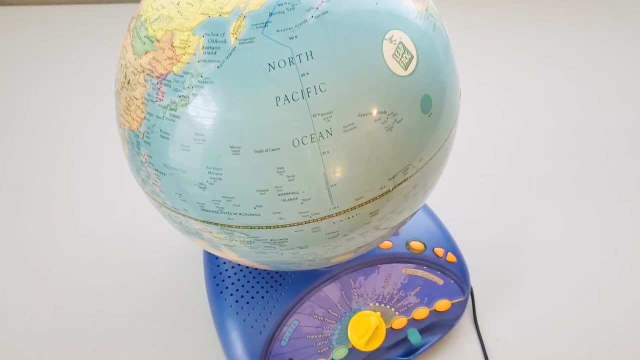 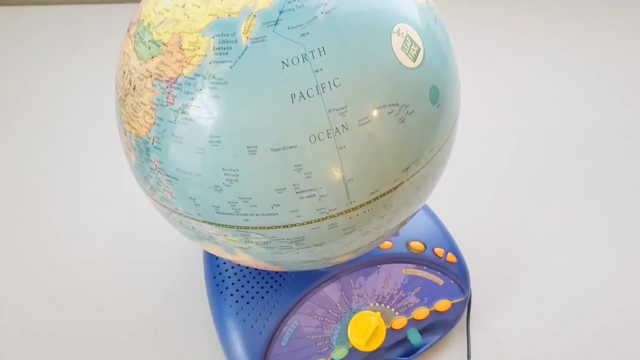 Try North. Look for the Arctic Ocean. I'm catching it. Why isn't it going? Can you find the Pacific Ocean? Find Africa. Eight continents or oceans found, Yay, Fantastic Round two. No, no, no, no. 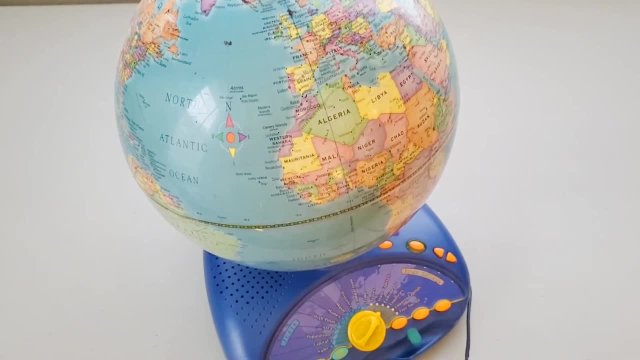 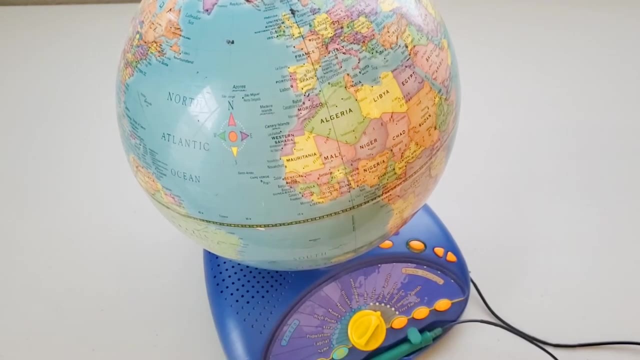 Press the. So that is how this interactive globe works. We haven't played with this in a while, so I kind of forgot how some of it worked, But this is a really cool resource to have on hand. I'm so glad I was able to find one. 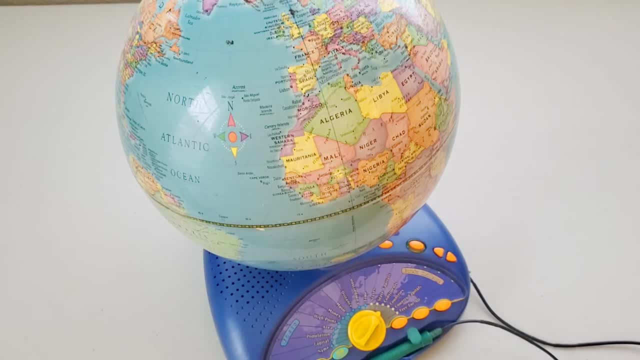 This is obviously an old version, so I will have to see if I can find either an updated version or maybe something similar from another brand, But I will link to something down in the description box if you want one of these for yourself. It's really cool. 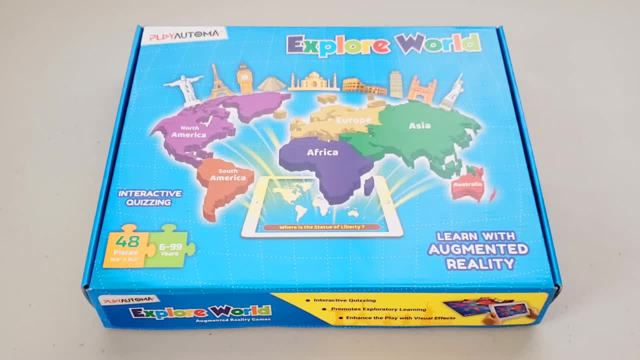 This next activity I'm going to show you was actually sent to me from the Play Automa brand, But the reason why I thought this was really cool was because I thought it was really cool to be able to play with this. I thought this was so cool in such perfect timing that this would be a really great resource. 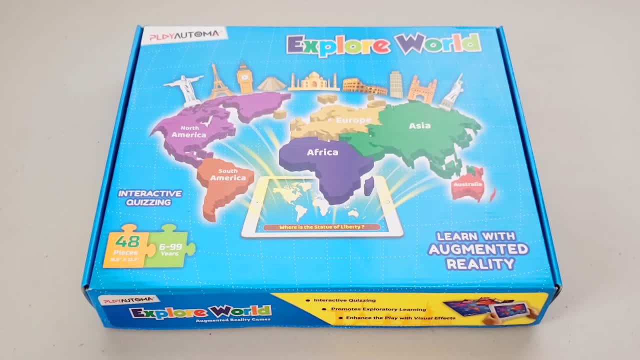 to use during this distance learning time. My middle child is currently learning about the countries and continents around the world, And he has to write two facts about each country every day, And the only resource he has been provided with is some YouTube videos, And it literally takes him hours. 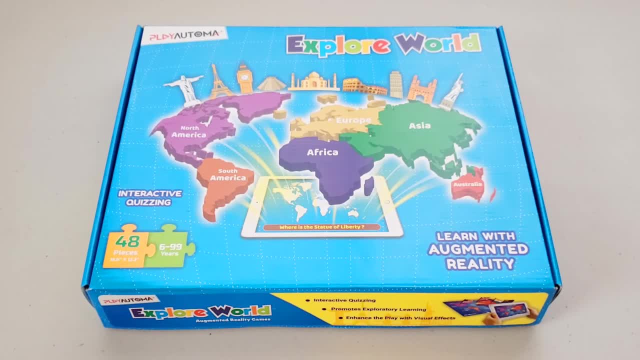 So I'm going to show you how to find facts on these countries. I don't know why it takes so long- It drives me nuts, And so this would be a really great activity to use for him, and he can easily learn the facts about all of these countries, continents, cities, whatever the case may be, landmarks. 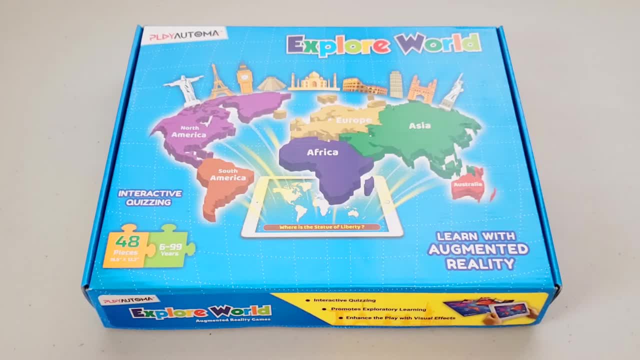 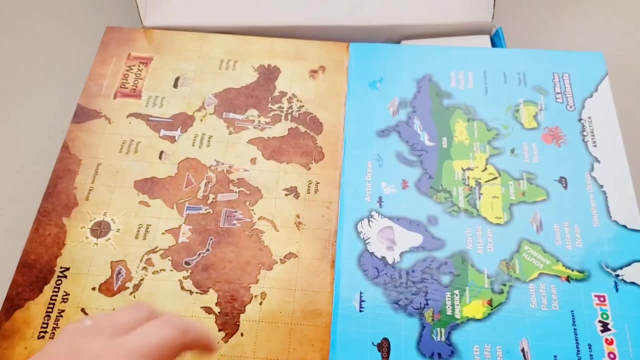 all of these things. So let me show you exactly how this thing works. It is so cool. So when you open up the box, you first have this really cool foldable map thing here. So it's hardcore, like sturdy material here. 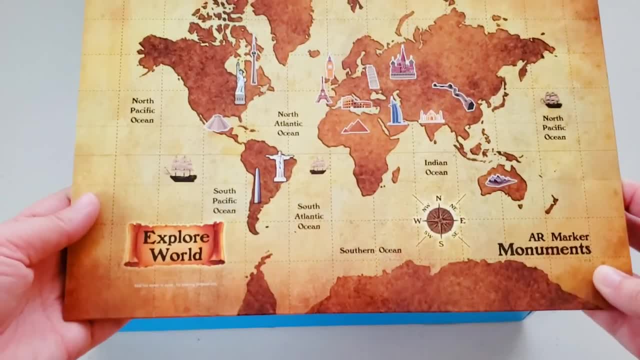 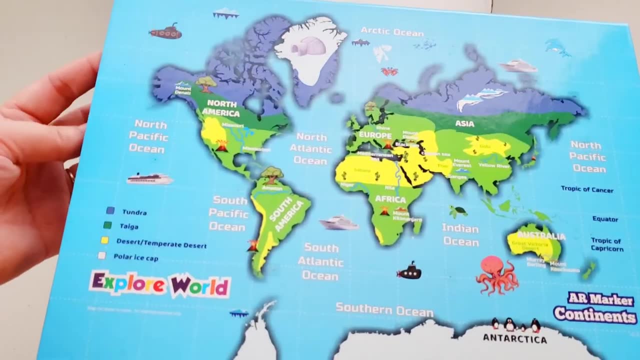 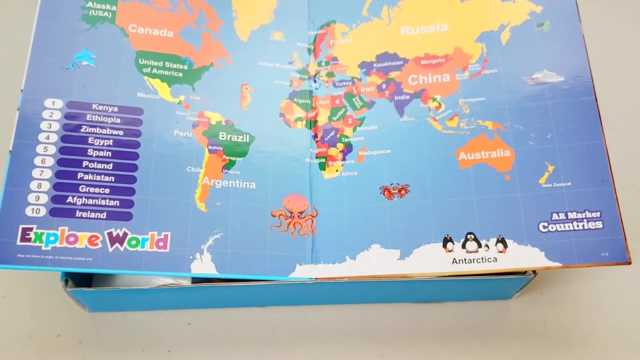 So on one side we have the landmarks or the monuments here as a display. On the other side we have the different continents, again basic information of what you can find there, And then on this side is a large picture of kind of the most popular, I would say, countries. 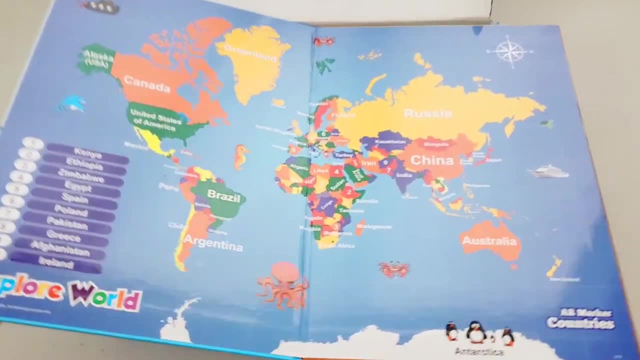 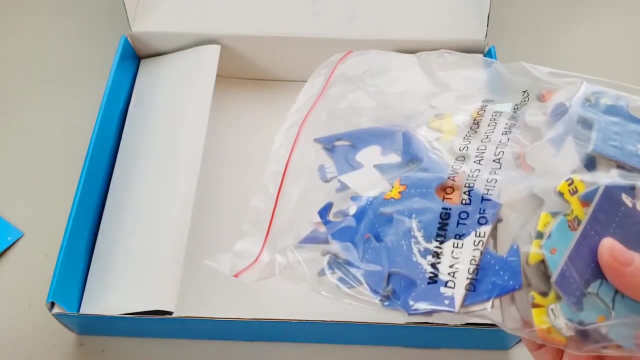 This is definitely not all of them, But this is like a basic view here. But the really cool thing about this is that you can find all of these things here, But the real part of this product is that this is actually a jigsaw puzzle. 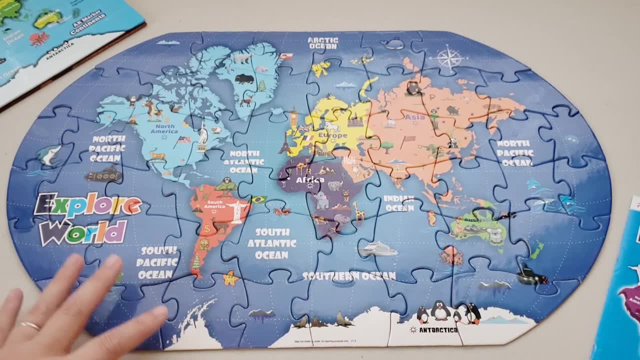 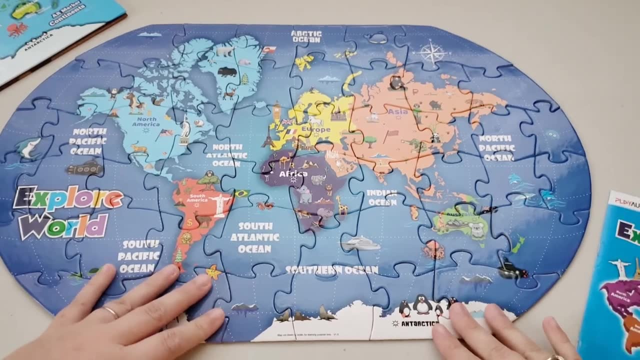 All right, so I have put the 48-piece jigsaw puzzle together Now. these are extremely thick puzzle pieces, so that's another plus to this thing. You don't really have to worry about your kids bending or breaking them. They could still chew on them. 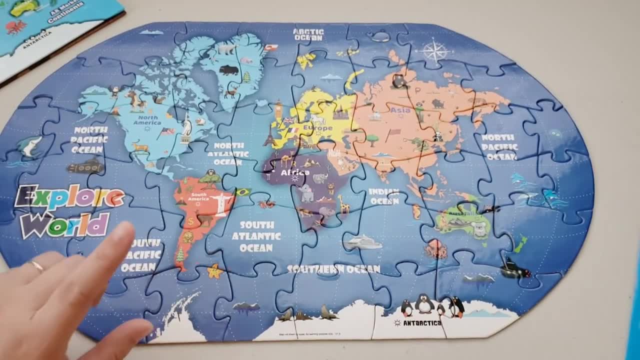 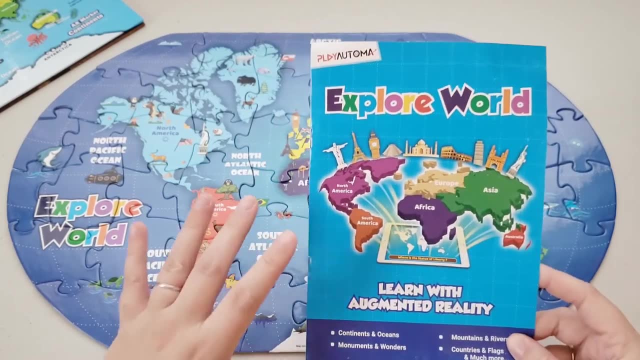 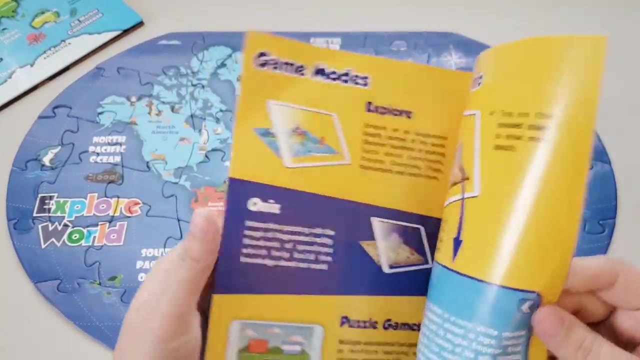 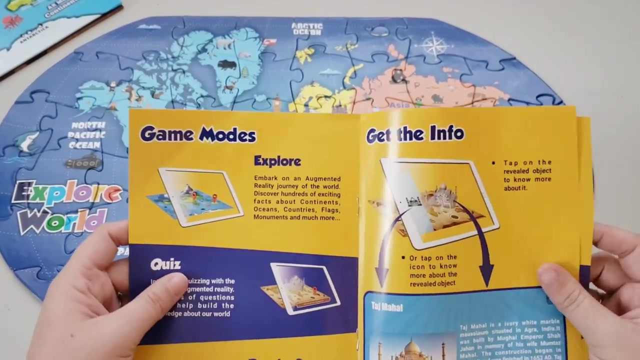 But they are very sturdy. so that's good. But what makes this jigsaw puzzle That much more interesting is that you can use your tablet to turn this into an augmented reality learning tool that brings the map to life. So, as you can see here in the pictures, it'll pop up different things on the map for you. 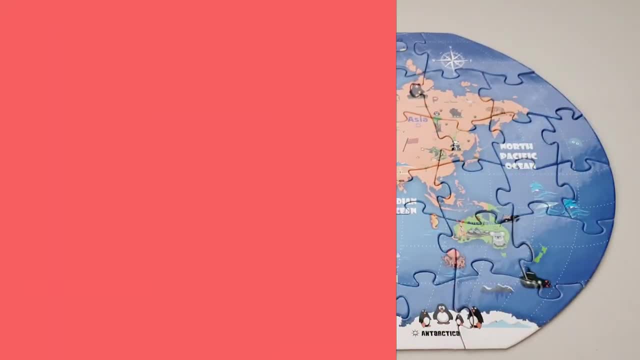 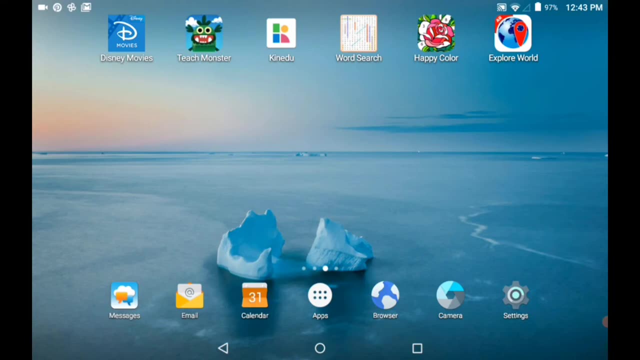 to then learn about. So let me get my tablet and show you how to work this thing. Okay, I have my tablet ready to go. This particular product does work with both Apple and Android, And I happen to have an Android little ridiculous tablet here. 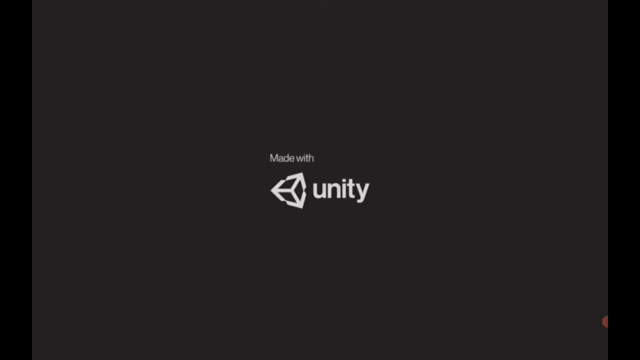 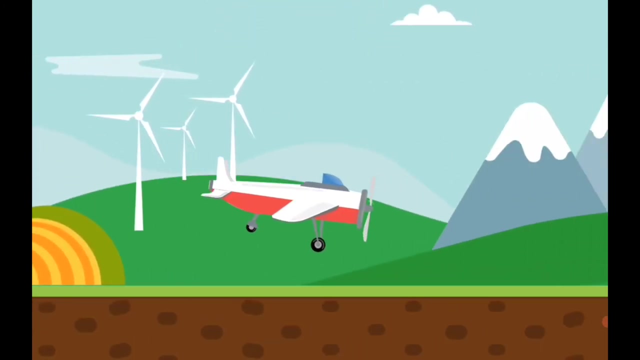 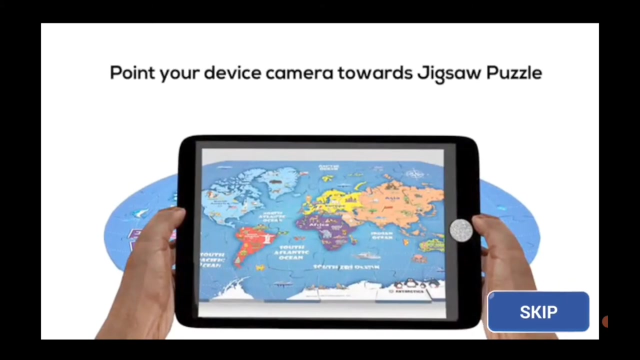 So the app is the Play Automa Explore World app. So now it's just showing you how to use the tablet and the puzzle together, which I will now do for you. So it's going to pull up a scanner here for you to scan the puzzle. 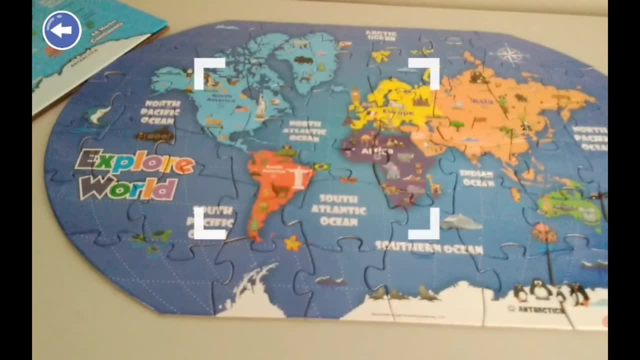 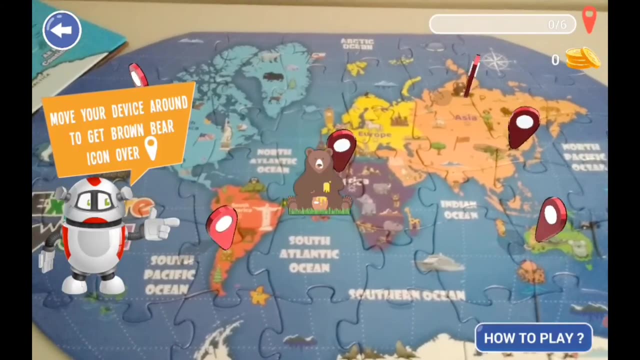 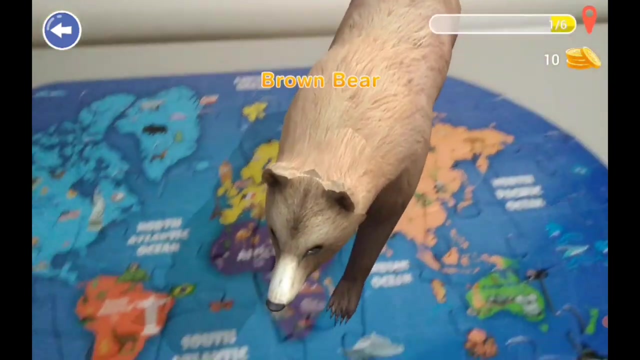 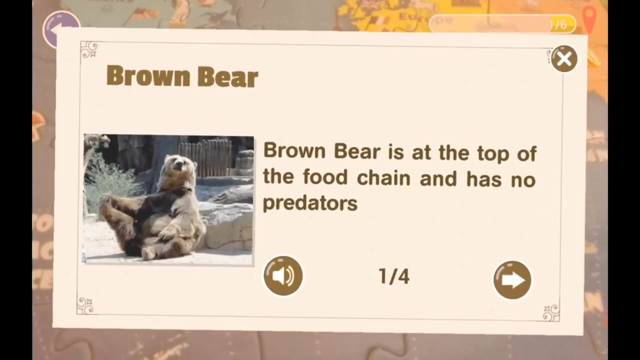 Let's see if I can do this. Now you're going to move your tablet around to where you would find the brown bear. Well done, You found brown bear. Now we're going to tap on the bear and learn some things about it. 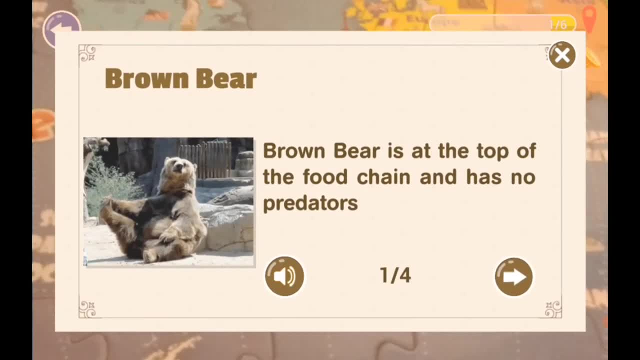 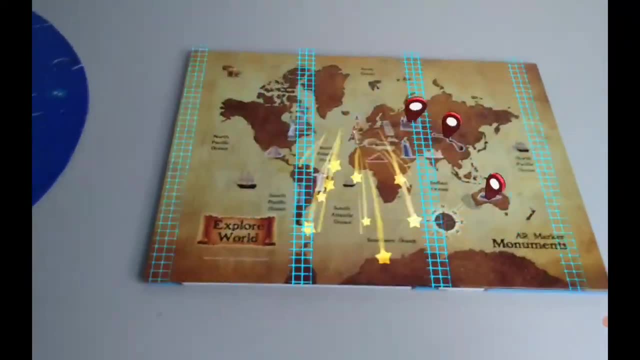 Brown bear is at the top of the food chain and has no predators. See how it's just simply giving facts. This would have helped my son so much, Just like with the jigsaw puzzle. now we're going to use the other board of maps to continue. 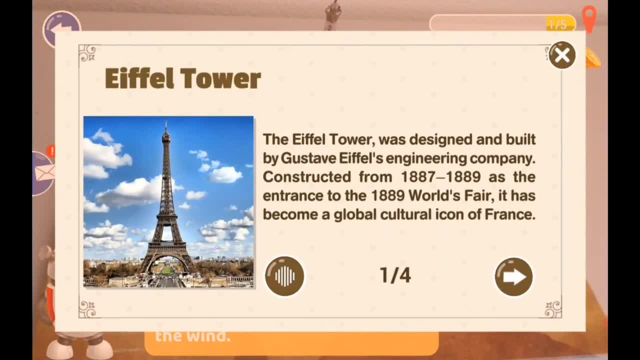 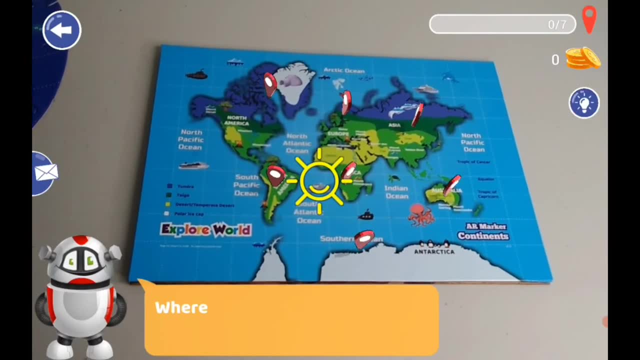 on throughout the game. So on here we're learning about the monuments. just click on them and learn a few facts. And then, on the next one, we're talking about the continents. Again, find them on the map and learn something interesting from there. 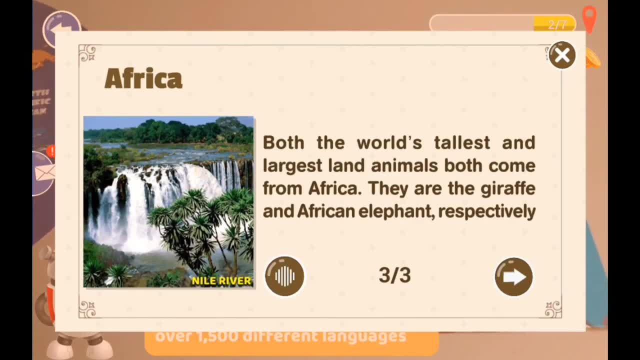 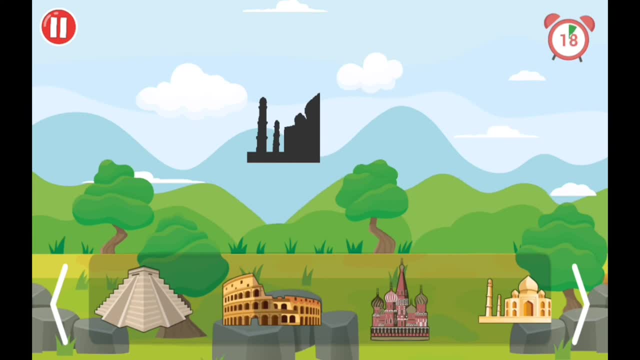 And then you also have the other side with the countries. So now we're going to apply this map on our board as well. With these you can earn coins to play mini games. So these are going to be trivia and review of what you have learned throughout using this game. So here we're doing kind of spatial. 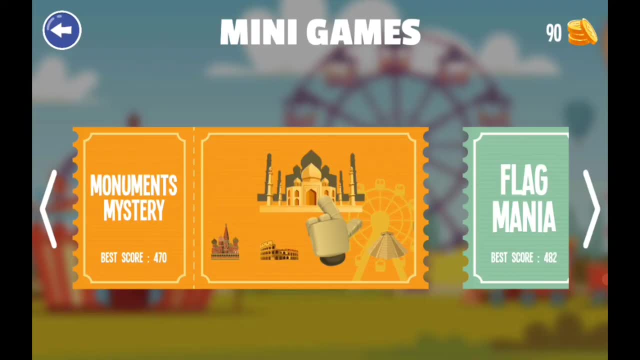 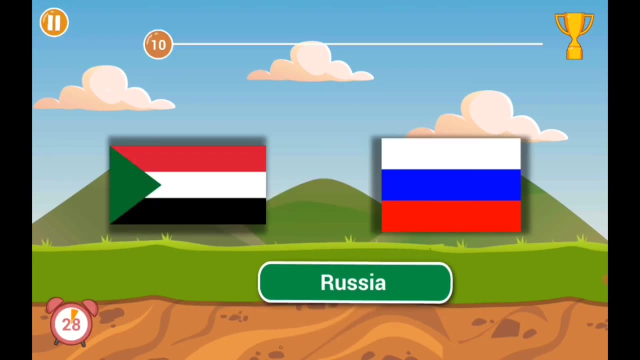 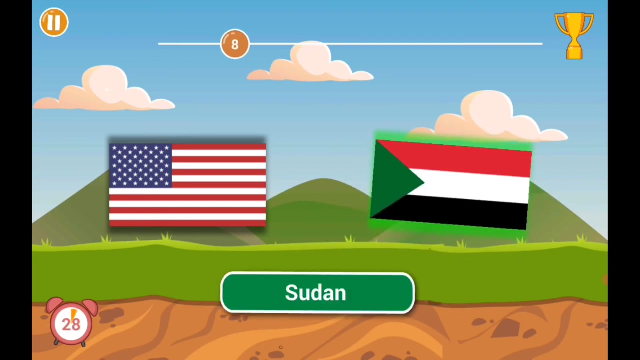 awareness memory type game. This one is flag mania, So we also learned about the flags for these different countries. This is one that even I missed a couple on, And I also did on the next game as well. So one thing about this particular product is that it is for ages 6 to 99. So even 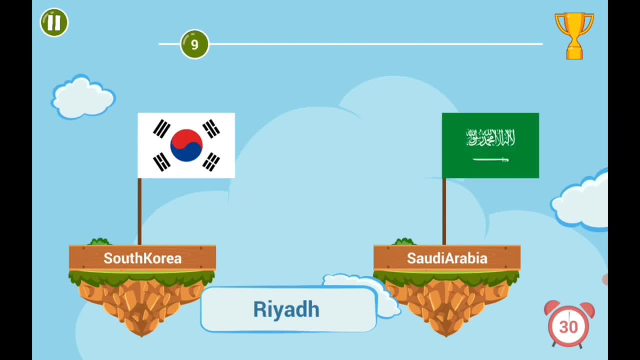 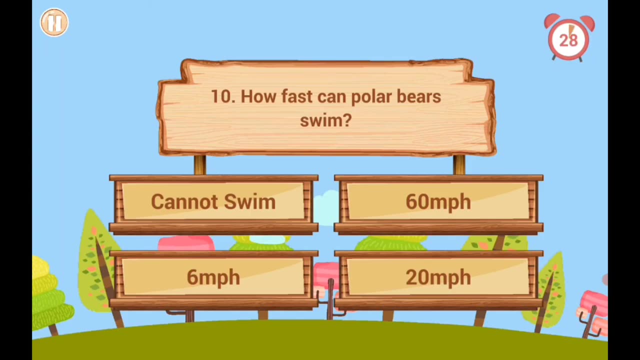 us adults can learn a thing or two throughout this game, So that's a lot of fun. And then the last mini game is going to be basic overall trivia that you would see in any other type of game like this. That is really interesting information, So I really highly. 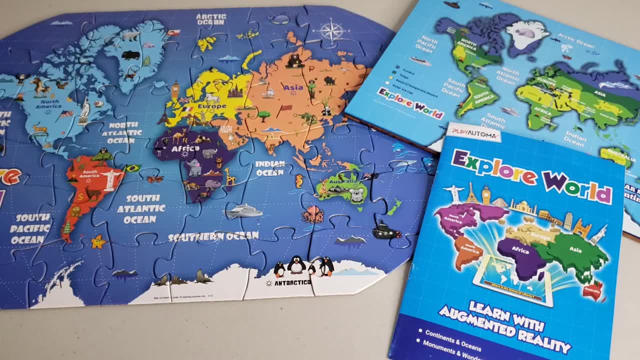 recommend it. If you're interested in this game, I highly recommend it. If you're interested in this game, I highly recommend this product. All right, everybody. I hope I was able to show you how cool this particular product is. I think being able to use your tablet to turn this into an 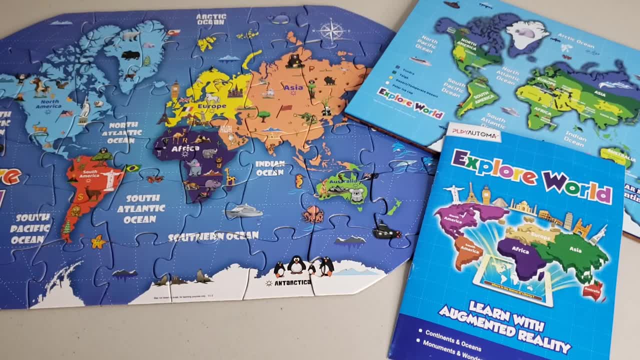 interactive puzzle and game and all these things is so cool. I really do think this is such a cool product, So thank you to Playautoma for sending it to us. It will have a link down below in the description box so that you can pick one up for yourself. I really think this is so cool. 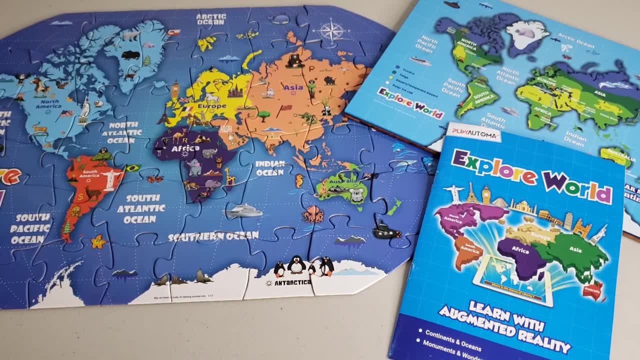 especially during these distance learning times, Since they're on their devices anyway, why not make it a little bit more fun and interesting by having some augmented reality? So cool. I hope you guys try out some of these activities to work with on your kids about world geography. If you like this video, give it a thumbs up. 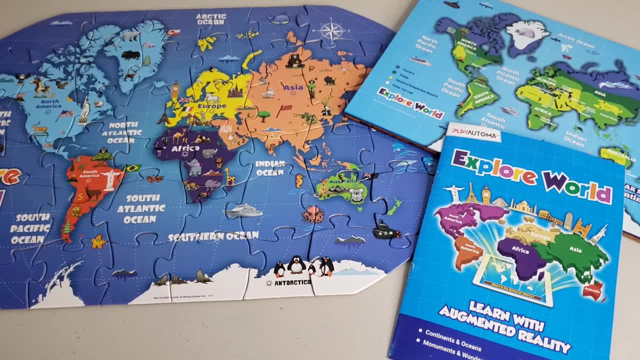 If you want to see more from me, then hit the red subscribe button and the notification bell and I will see you guys in the next video. Thanks for watching. Bye.